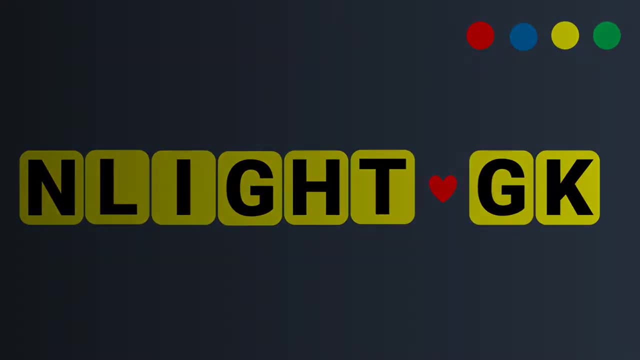 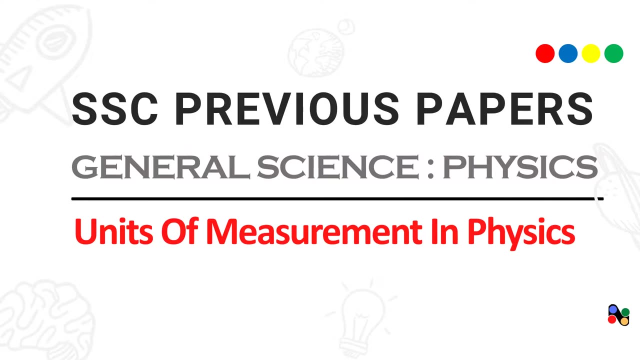 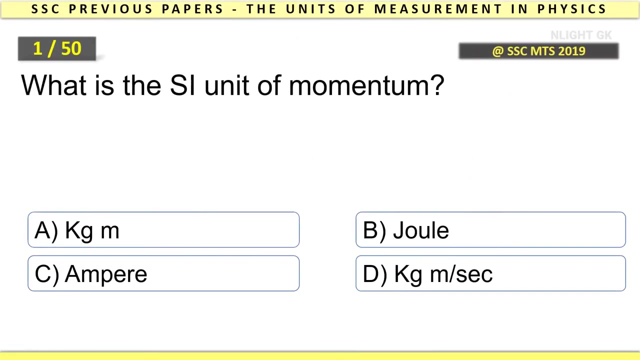 In this video you will be listening to the important questions from the units of measurement in physics that is being asked repeatedly in various exams of SSC. For more parts, find the link above or from the description. What is the SI? unit of momentum. 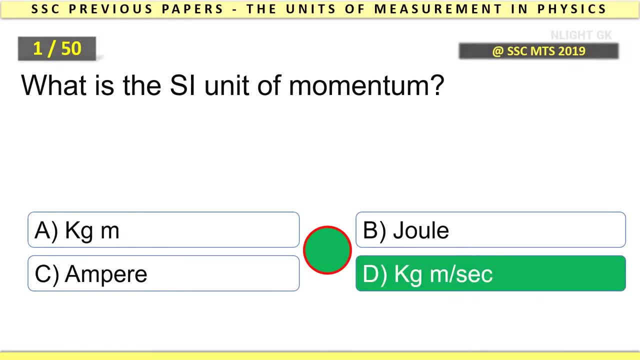 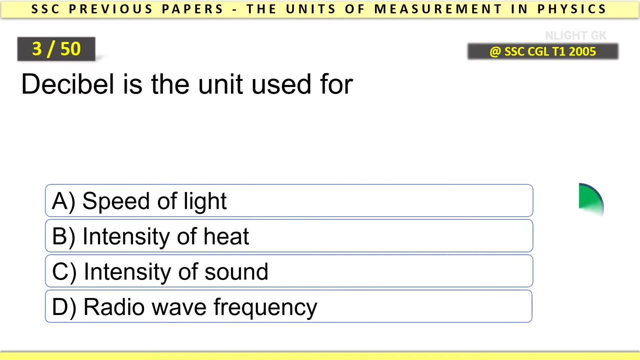 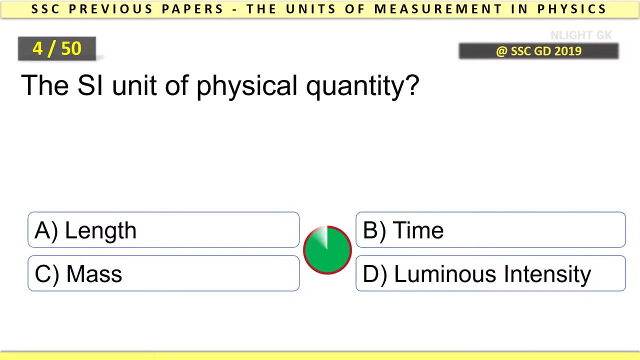 Kilogram meter per second. The SI unit of radioactivity is Becquerel. Decibel is the unit used for Intensity of sound. The SI unit of physical quantity, Mass Energy in the foods- can be measured. in which units? 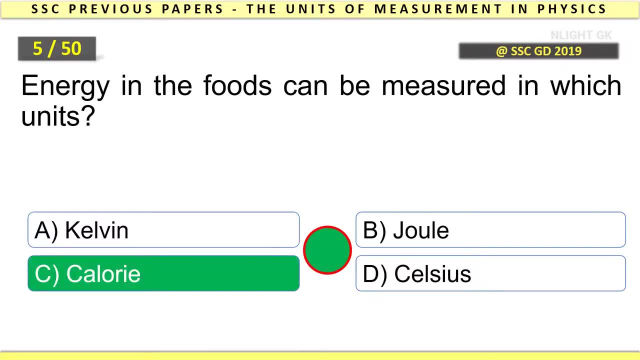 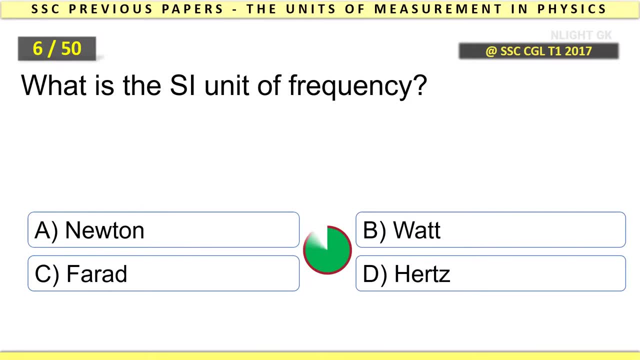 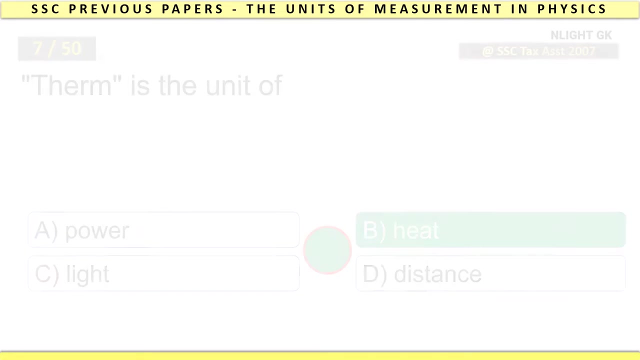 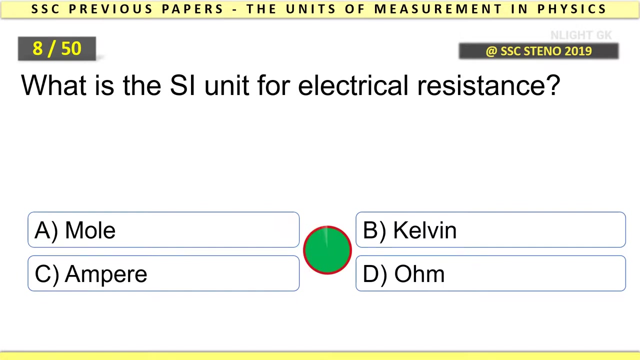 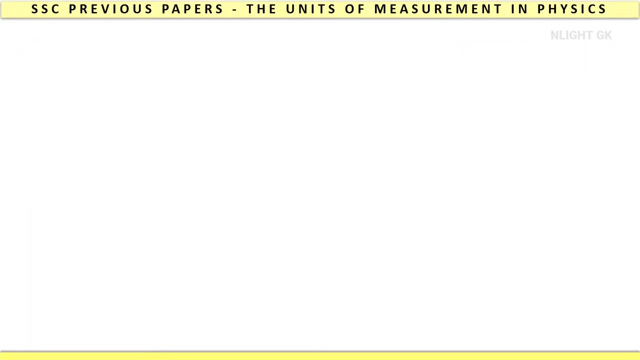 Calorie. What is the SI unit of frequency? Hertz Thumb is the unit of Heat. What is the SI unit for electrical resistance? Ohm Ferad is the unit of Capacitance. Which of the following physical quantity SI unit pairs? 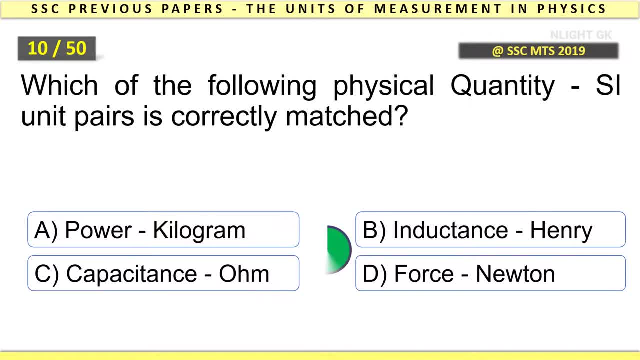 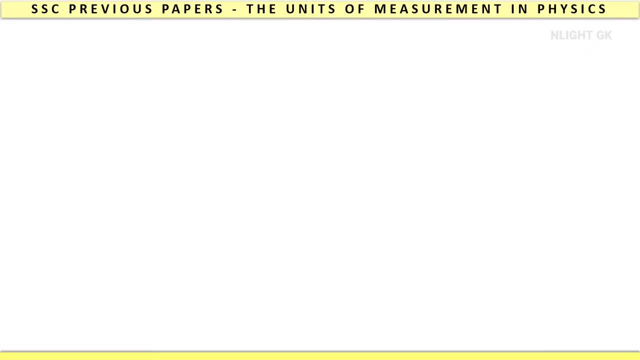 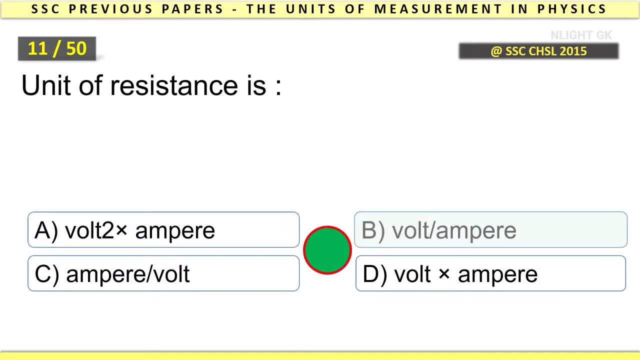 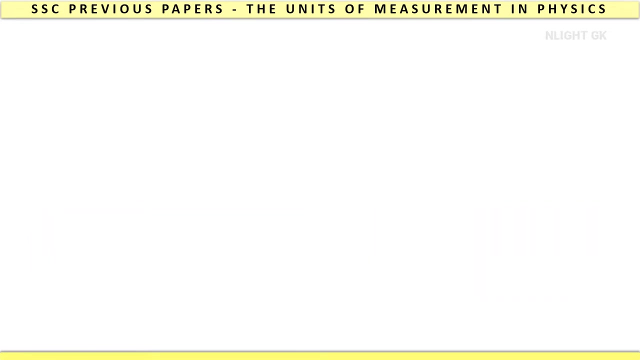 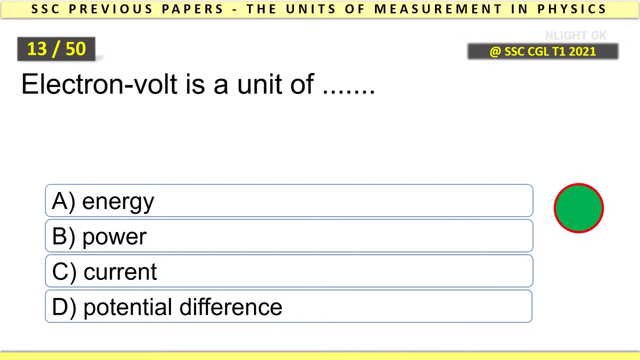 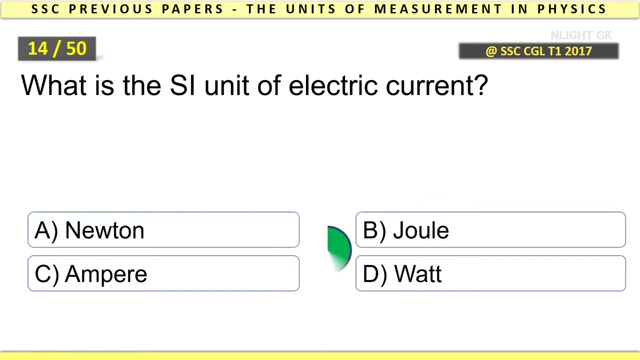 SI unit pairs this correctly matched Force. Newton Unit of resistance is Volt per ampere. A light here is a unit of Distance. Electron volt is a unit of Energy. What is the SI unit of electric current, Ampere. 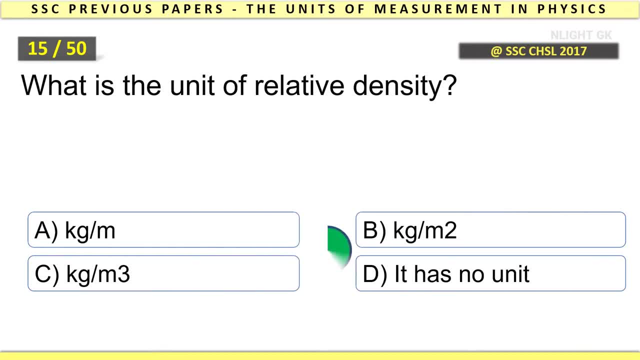 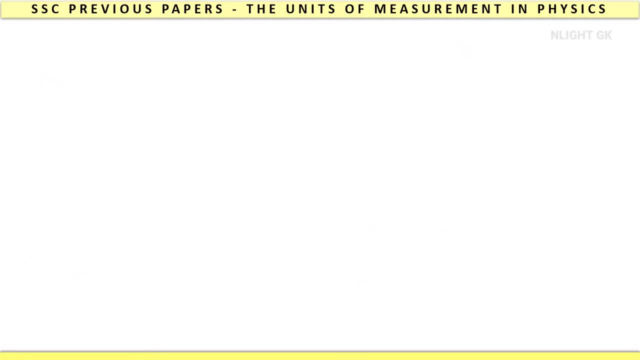 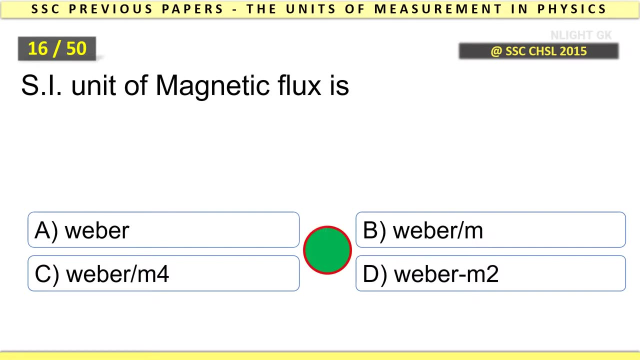 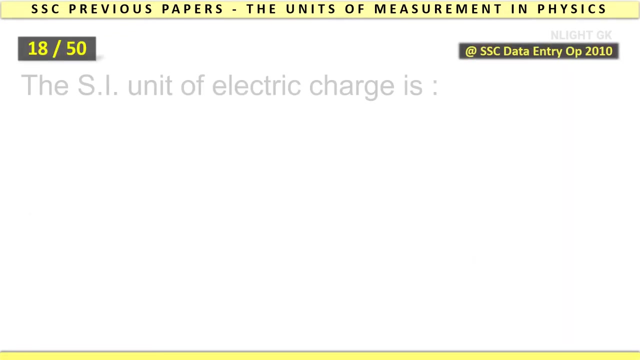 What is the unit of relative density? It is a unit of relative density. It is a unit of relative density. It has no unit SI unit of magnetic flux is Weber. What is the SI unit of power? Watt? The SI unit of electric charges. 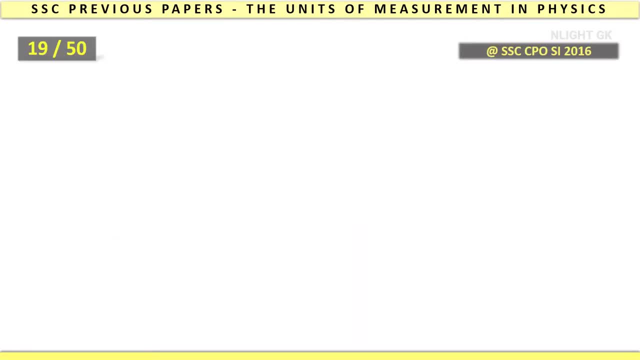 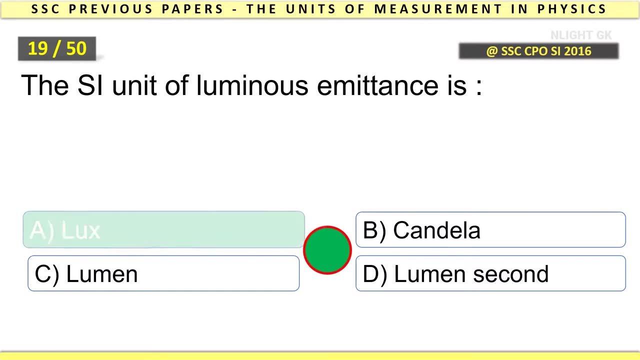 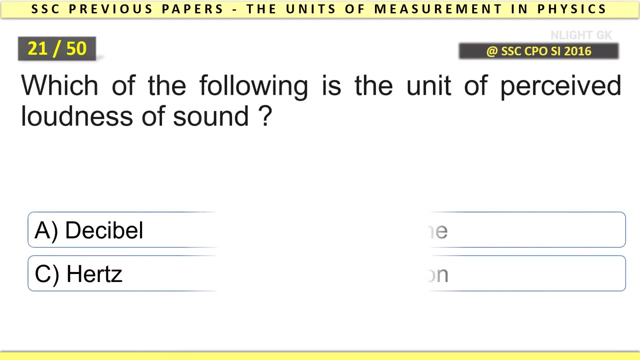 Coulomb, The SI unit of luminous emittances, Lux. What is the SI unit of heat energy, Joule? Which of the following is the unit of perceived loudness of sound? SONY. The important unit of a microprocessor is: 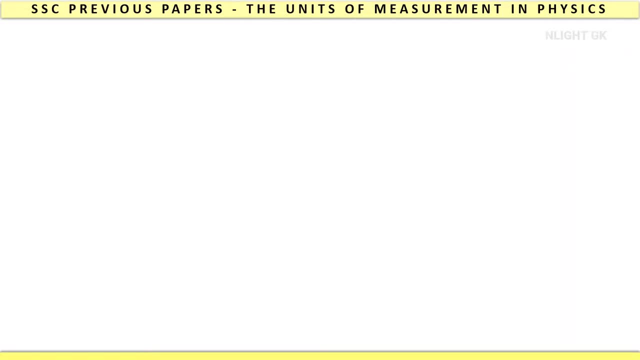 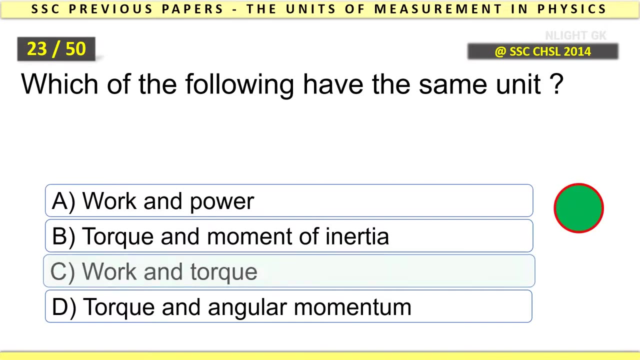 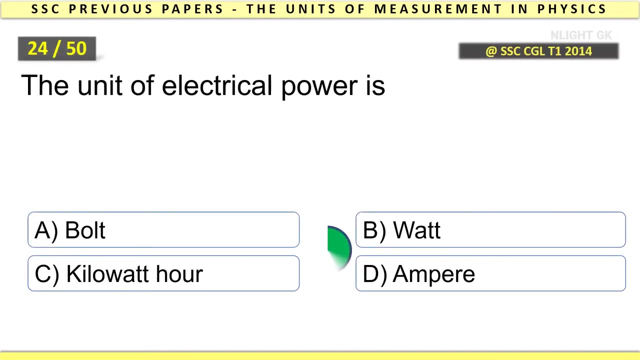 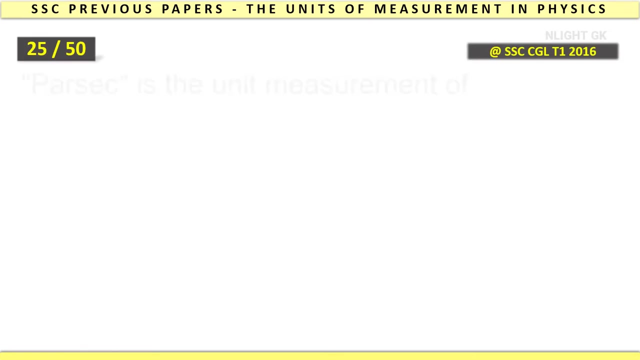 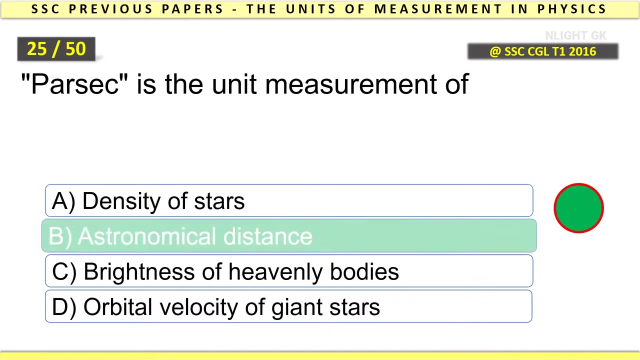 All of the above? Which of the following have the same unit? Walk and talk. The unit of electrical power is SONY. The unit of electrical power is Bolt Bolt. Parsec is the unit measurement of Astronomical distance. 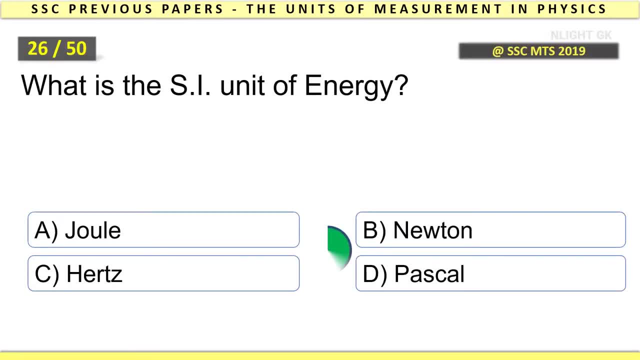 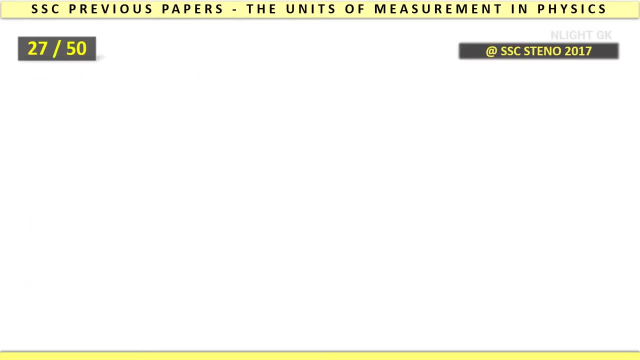 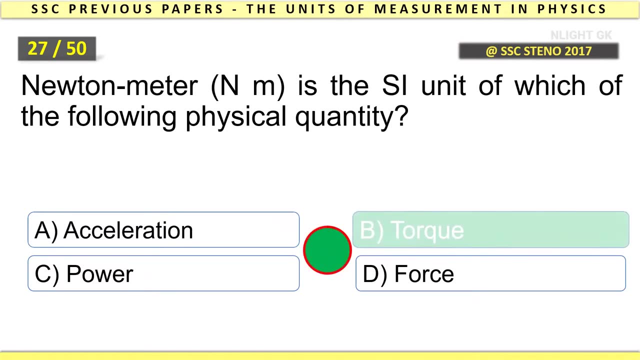 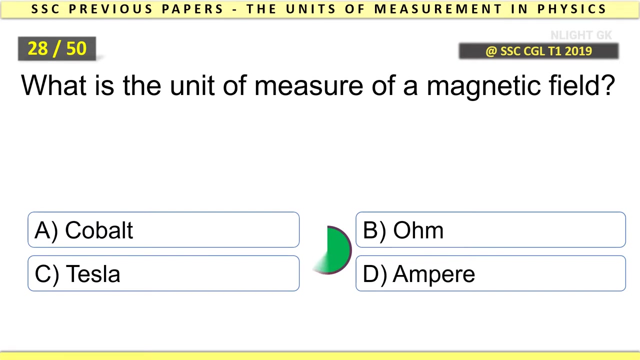 What is the SI unit of energy? Joule, Newton, meter? is the SI unit of which of the following physical quantities: Quantity, Torque. What is the unit of measure of a magnetic field? Tesla? What is the SI unit of pressure? 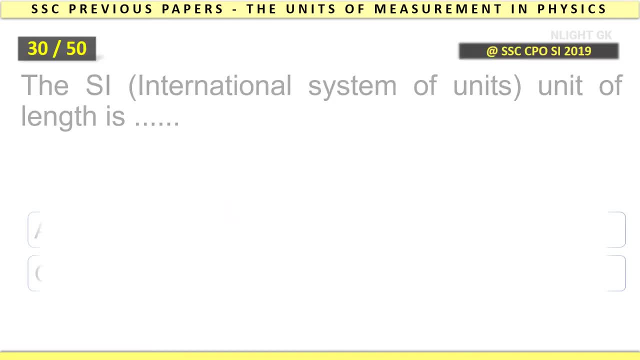 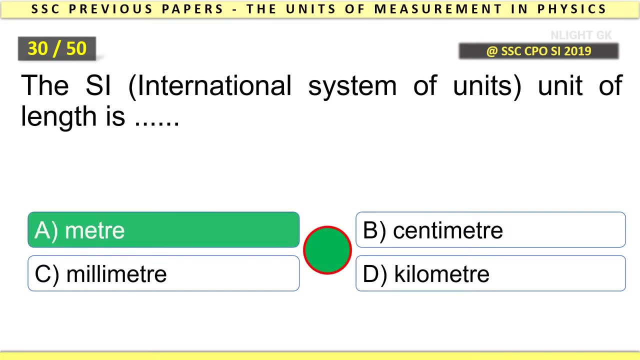 Pascal. The SI International System of Units is the unit of pressure of a magnetic field. The SI International System of Units is the unit of pressure of a magnetic field. Pascal, What is the unit of length is Meter? Curie is a unit of. 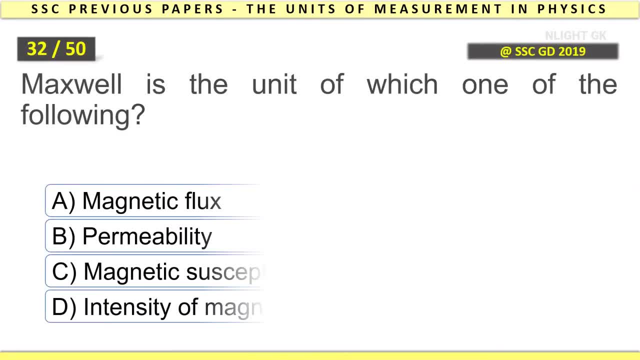 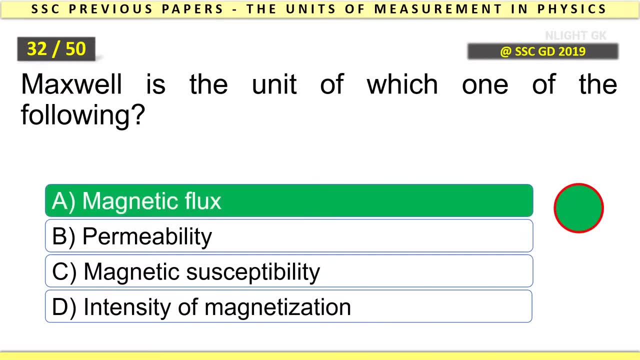 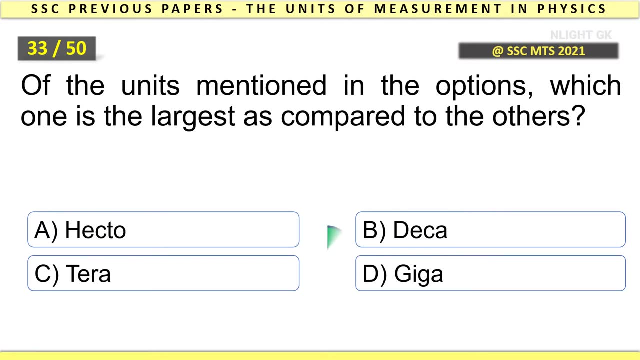 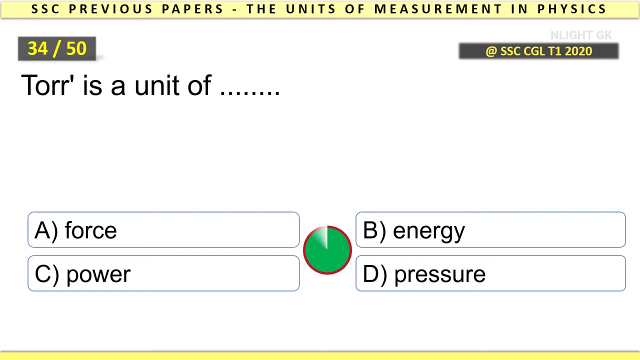 Radioactivity. Maxwell is the unit of which one of the following Magnetic flux. Of the units mentioned in the options, which one is the largest as compared to the others? Tera Tor is a unit of Pressure. Weber is the unit of. 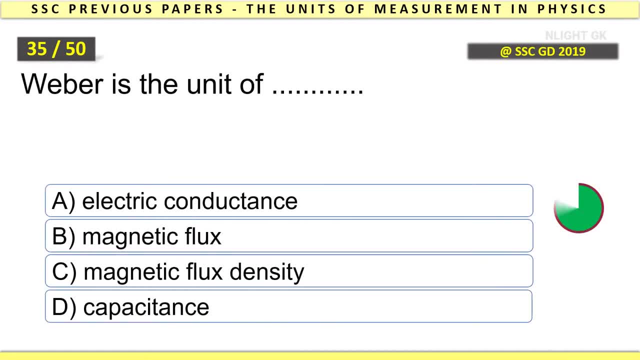 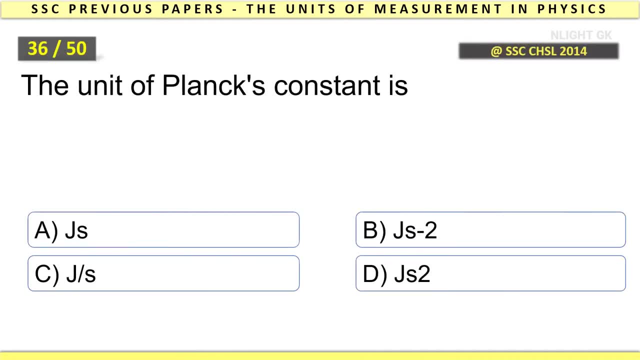 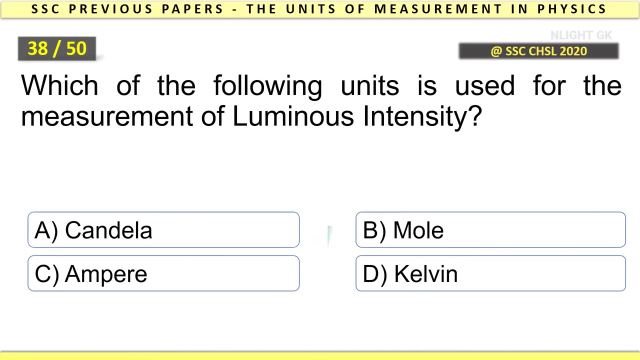 Tera Magnetic flux. The unit of Planck's constant is Joule. second Photon is the fundamental unit. quantum of Light: Which of the following units is used for the measurement of luminous intensity? Light A light here is a unit of. 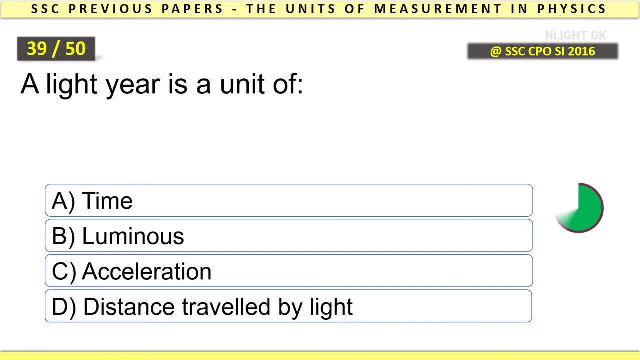 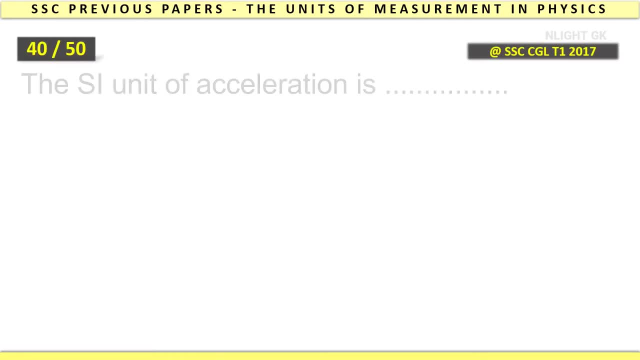 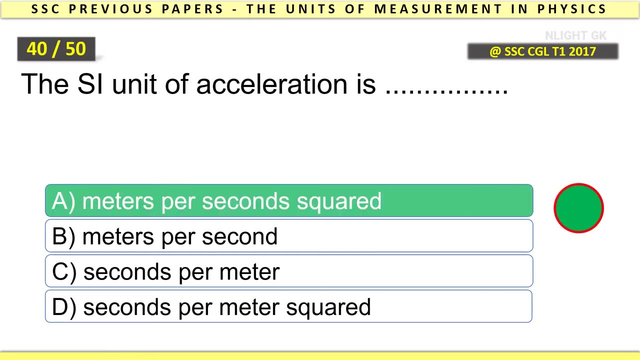 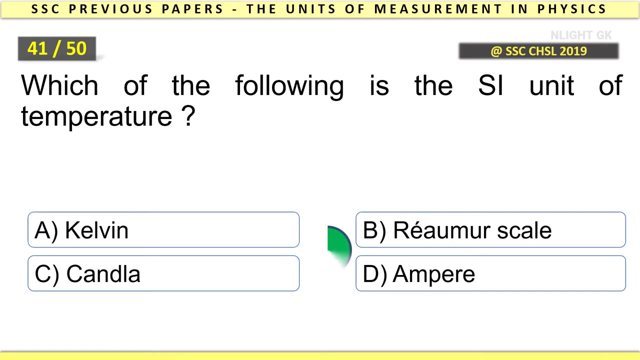 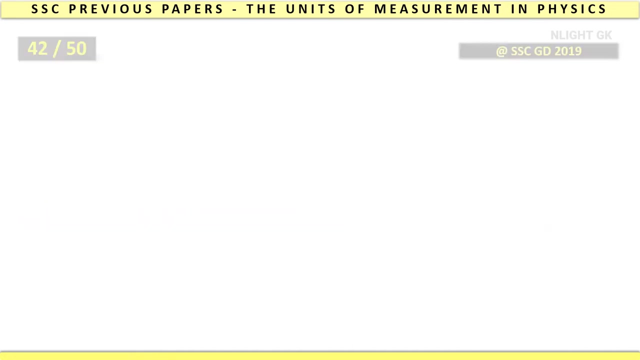 Candela A light. here is a unit of Distance travelled by light. The SI unit of acceleration is Metres per second squared. Which of the following is the SI unit of temperature? Tera, Tera Kelvin? Identify the SI unit of electrical resistance. 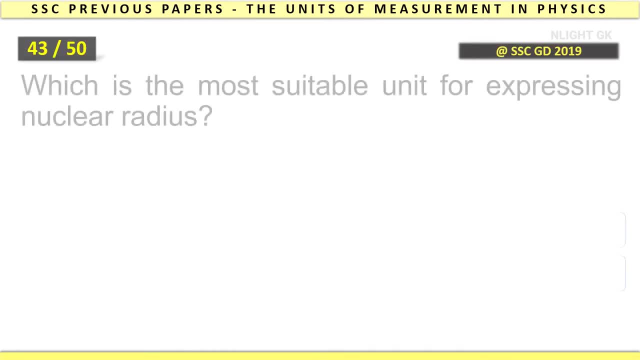 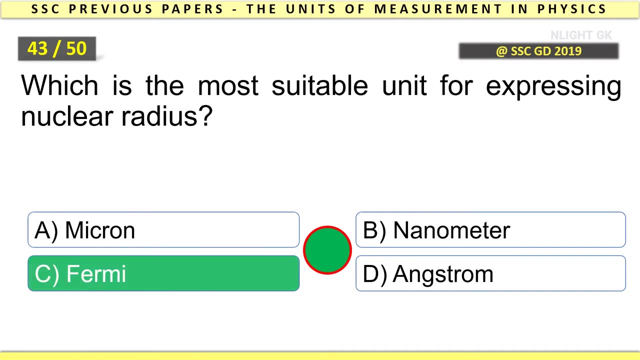 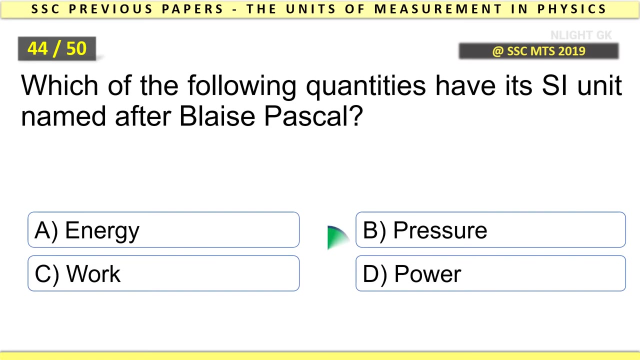 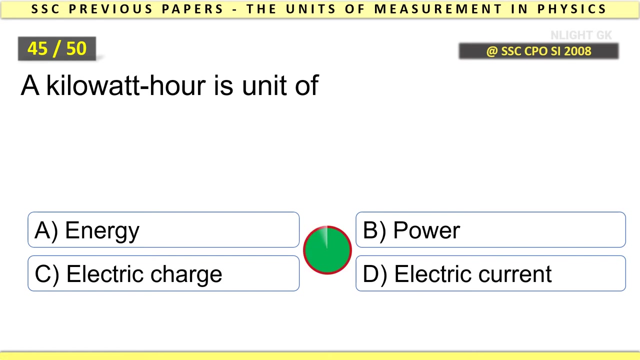 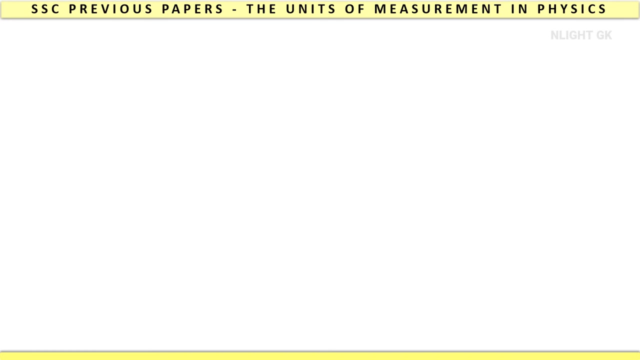 Ohm, Which is the most suitable unit for expressing nuclear radials? Fermi. Which of the following quantities have its SI unit named after Blaise Pascal? Pressure A kilo Watt hour is unit of Energy. Hertz is the SI unit of Frequency. What is the unit of calorific value?